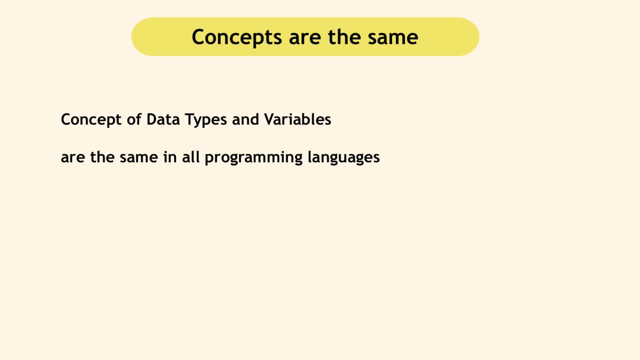 So if I was doing a Java tutorial, the concepts will be the same. The difference is in the syntax, And this is a good thing, because, unlike learning natural languages, when you learn one programming language, it will be much easier to learn another one. 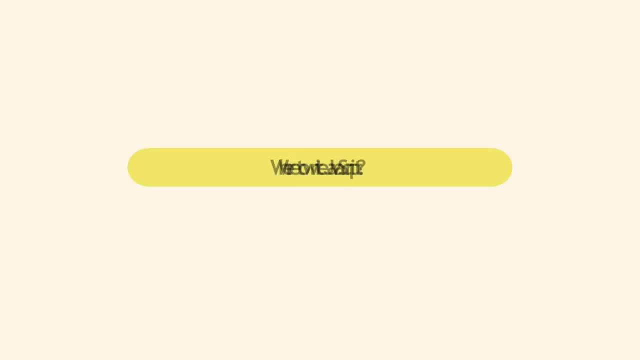 So, with that said, let's dive right in Now. the simplest way to start writing JavaScript is directly into the browser, Since, as I mentioned in the previous video, all modern browsers are able to interpret JavaScript and come packaged with so-called developer tools. 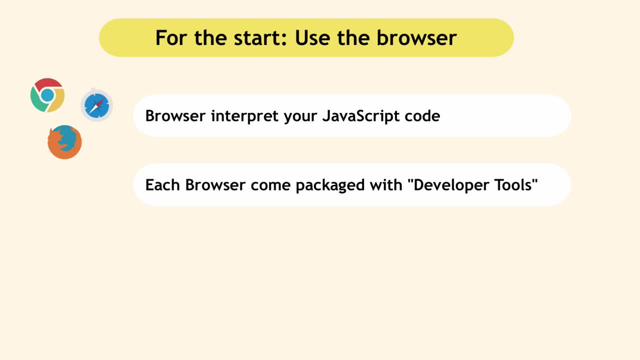 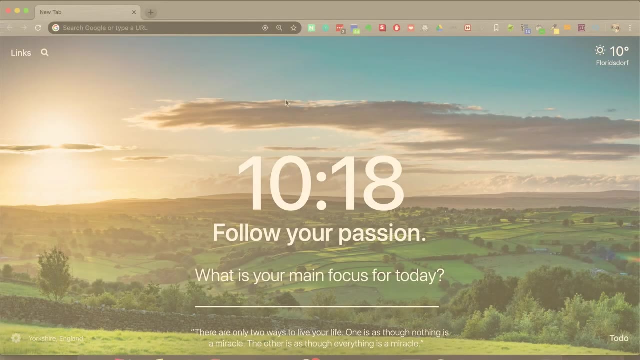 So open I The Firefox or Chrome browser on your laptop. if you don't have these browsers installed, I suggest you install them, because using browsers like Internet Explorer to run and execute JavaScript is not a good idea. So I would download either Firefox or Chrome and, in your browser, right click somewhere on the surface. 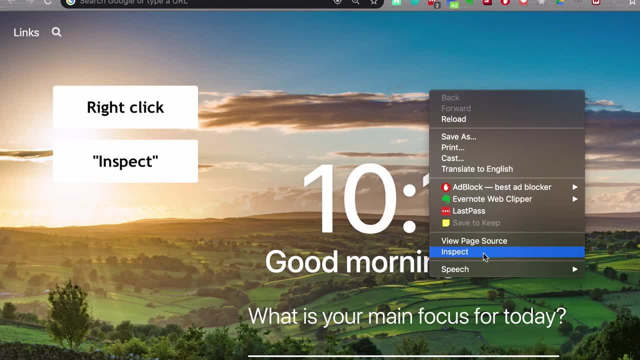 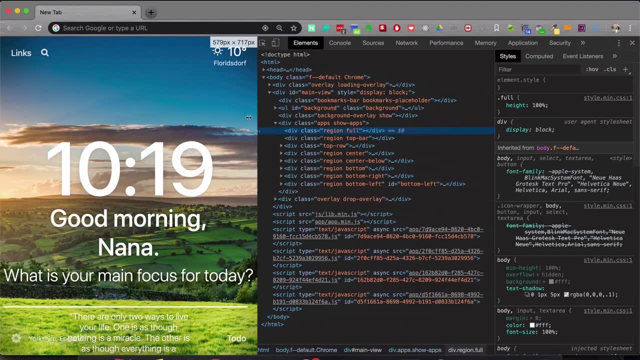 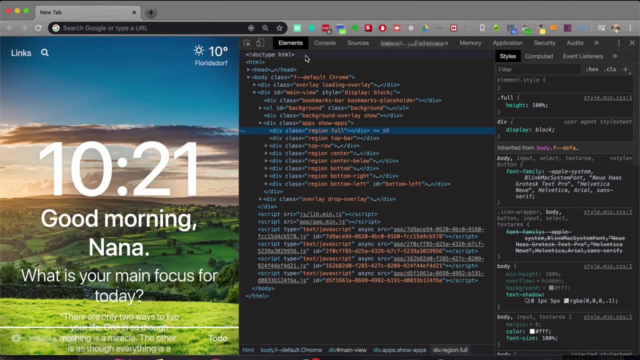 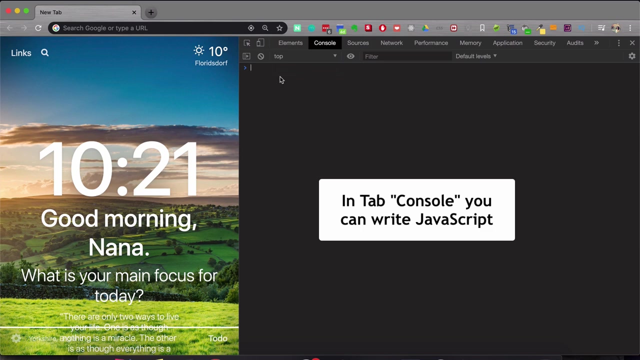 And select inspect. if your browser is in your native language then it would be called something else, but it should translate to inspect and when you click that you see something like this: And this space right here is called developer tools And here you should see a console tap and when you click on it you get this space where you can write JavaScript directly in the next video. 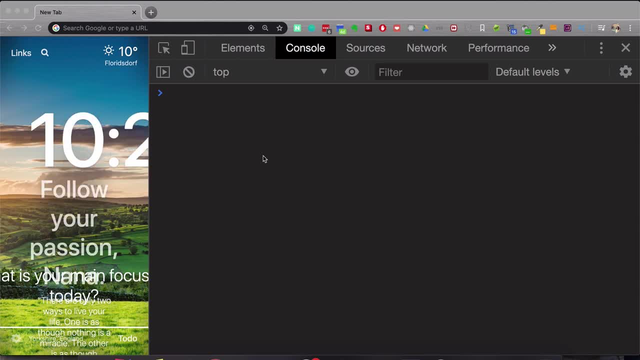 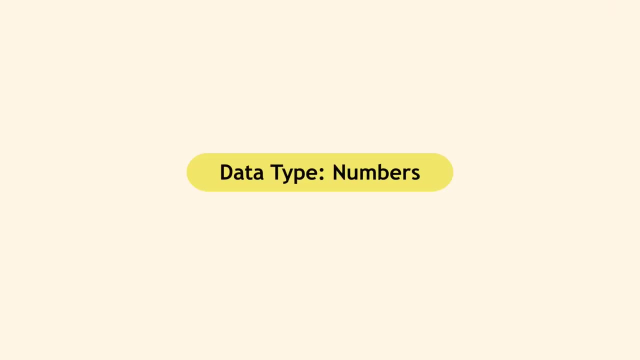 I will show you all the different places where you can write and execute JavaScript and which one you will usually use as a developer, But in this video we're going to use the browser console so that I can demonstrate some simple Examples. so the first data type that we're going to talk about is numbers. 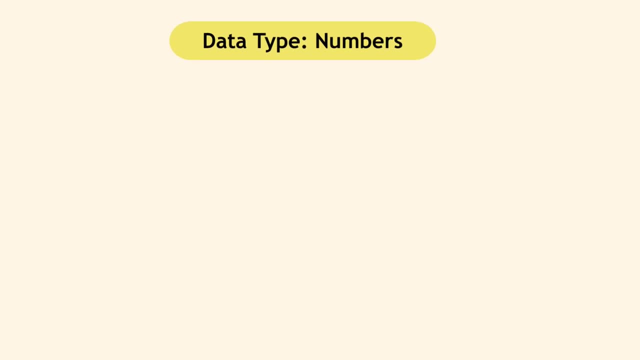 Obviously, when you're writing an application, you need numbers. Some of the examples are: YouTube displays number of subscribers for each channel, or number of likes for each video, or how many videos one has. When you search something on a Web application like Google, for example, you usually see total hits, et cetera. 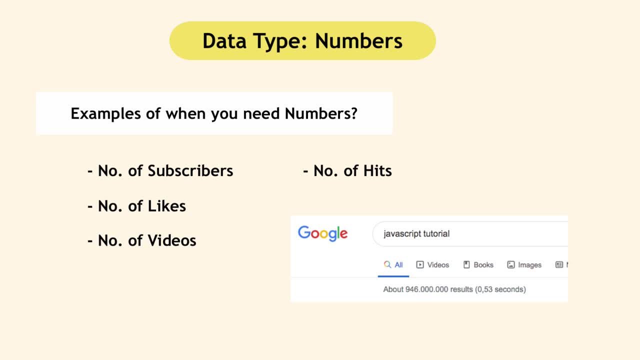 So these are all use cases where you need numbers and these examples Use whole numbers. But, for example, when you have an online shop where you need to display prices, prices obviously won't be whole numbers always, but rather decimal numbers with same precision. 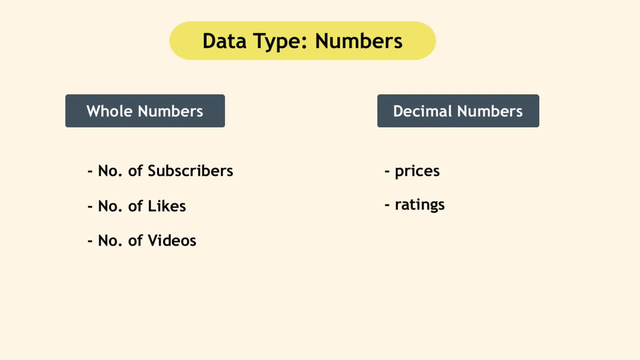 Also Amazon ratings. right, They can be four point five, for example, and in JavaScript their own data types for whole numbers and for decimal numbers. The whole number data type is called integer and these are numbers like zero, three hundred minus forty five. 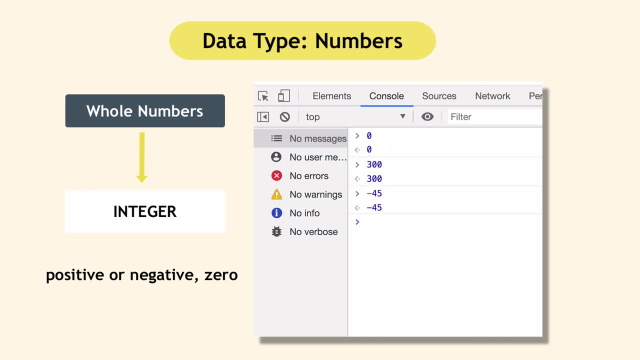 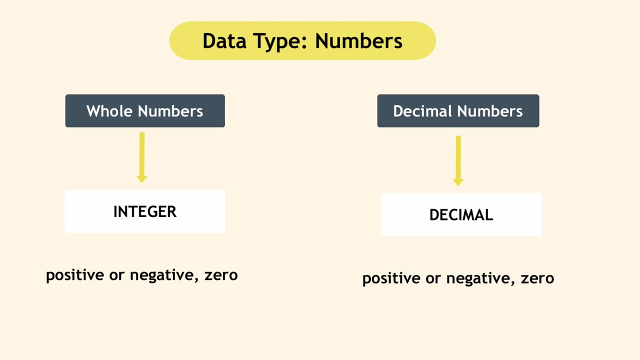 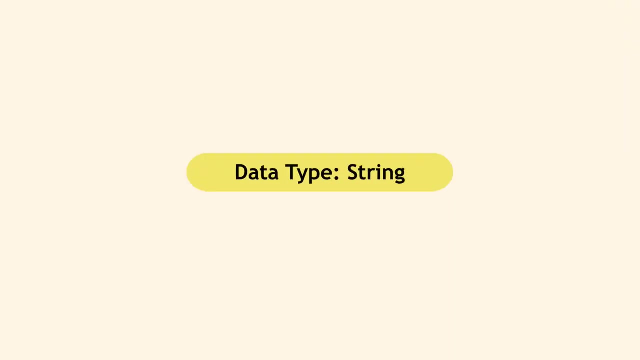 So positive, Negative numbers, they're all integers, and decimal numbers have a data type of decimal And again they're positive or negative or zero, zero point zero. ninety point seven hundred seventy seven minus fifty point five. They're all decimals. The second data type is string. 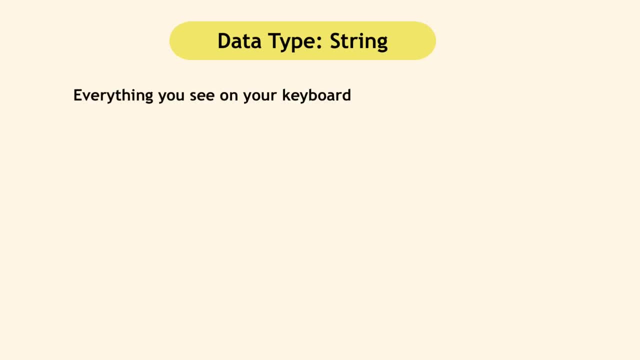 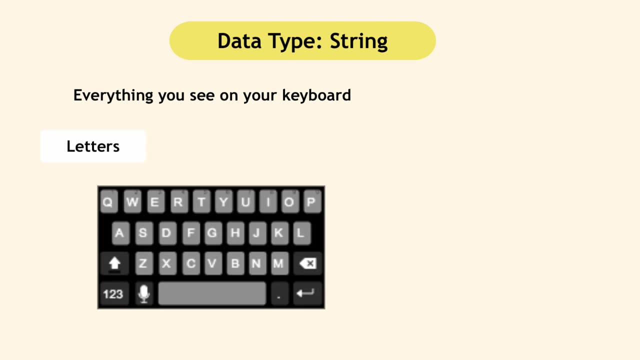 The way I like to explain what string is is basically everything you see on your keyboard. So obviously all the letters, no matter what language they're in, but also the special characters like ampersand, percent plus, minus and also the space character on a keyboard. 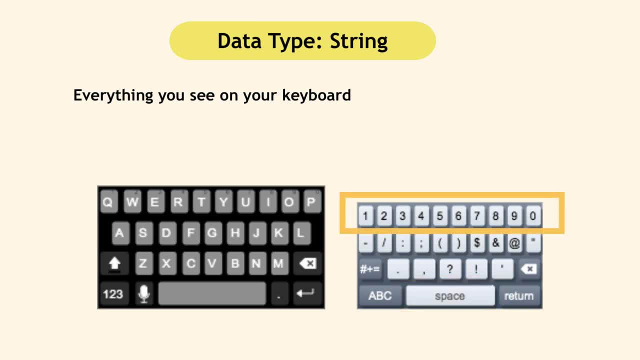 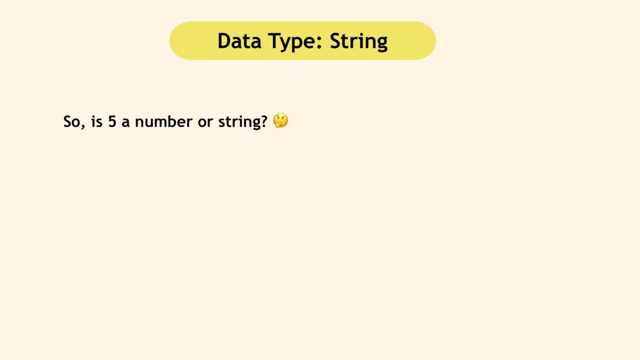 You also have numbers, and numbers are characters or strings also. So how does JavaScript know whether you mean a number, like integer, or decimal, like five, for example, or a character five? It knows it using quotes, So you tell JavaScript that you're using. 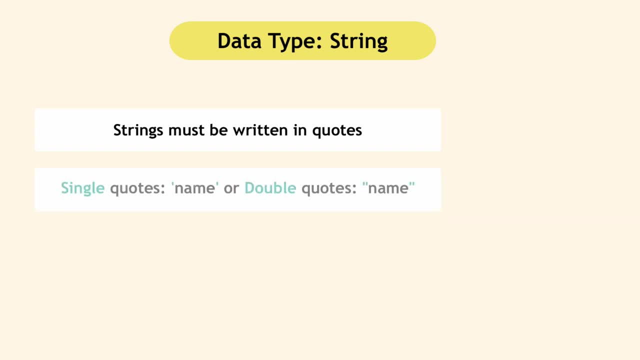 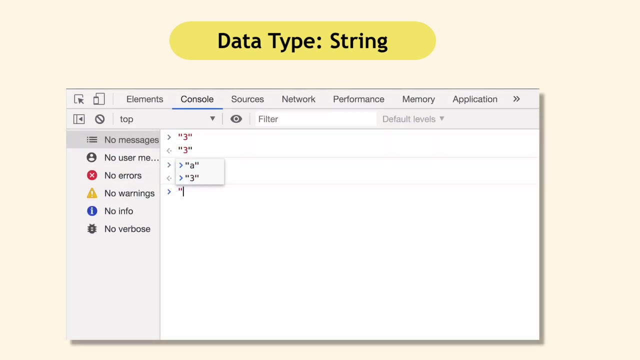 String by using quotes could be single quotes or double quotes, So these single characters or any combination of them is a string. So let's say a couple of examples, So three in quotes is a string: A with umlauts, letters from non English alphabets, combination of letters and numbers, special characters like an email or in password, and also an. 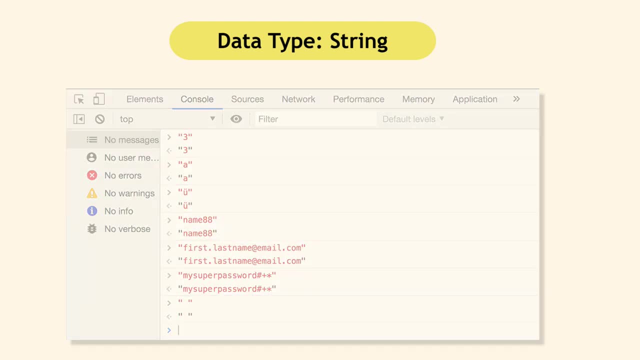 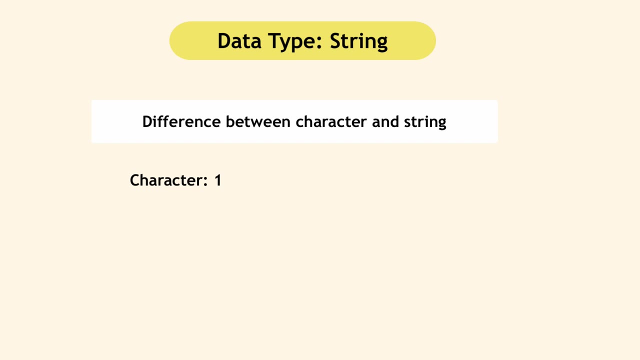 Empty space. character is also a string. So just to mention here. so difference between character and string. So character is basically just one letter or one number, one special character, and string is a character or a combination of multiple characters. So these are all strings and this single keys are characters. 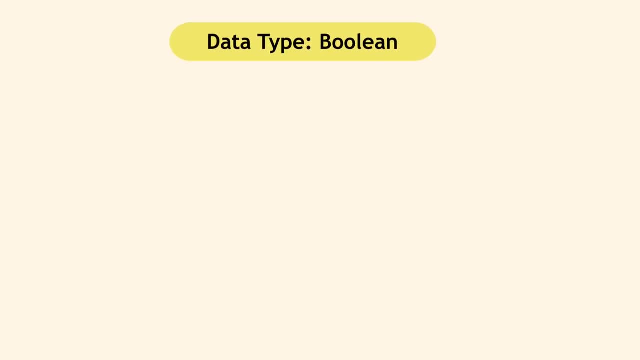 Another data type in programming languages is Boolean. Now to understand this, let's say you enter wrong password when logging into your application. Usually you get a message saying you provided a wrong password. or you accidentally enter wrong credit card number when buying tickets, or invalid email address when registering. 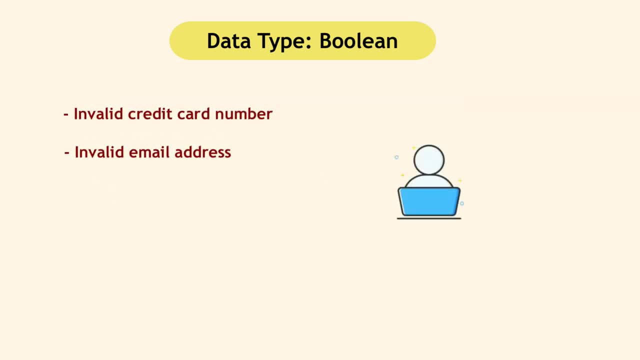 So in the background, developers write JavaScript code that validates whether the information that you provided is wrong or right or correct, And to express That wrong or correct state booleans are used. So word true expresses correct state and false expresses wrong state. So again, 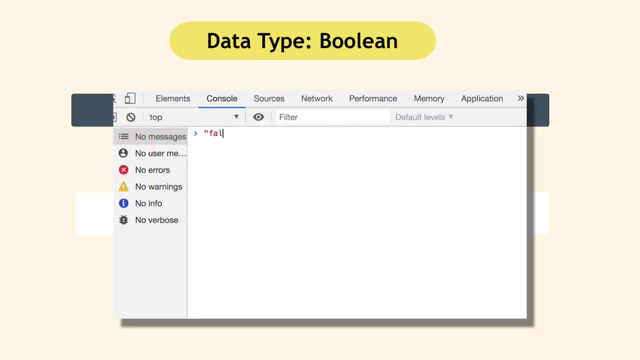 just like with numbers. you can write a simple string, false- with quotes, and JavaScript know that you mean a string without quotes. It will be a Boolean expression: false. That's how JavaScript can differentiate between those two. In addition to that, true, false can also be used for simple. 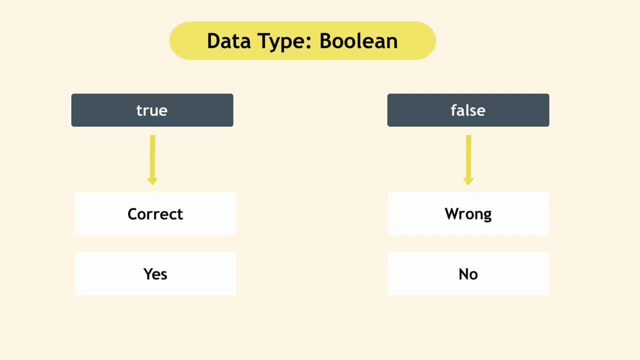 Yes, no. situations like: is the apartment on Airbnb available to book on this date? Yes, no, that will be true or false in Boolean terms. or is user logged in? depending on whether logged in or not, You will see different web page. That's a Boolean expression. 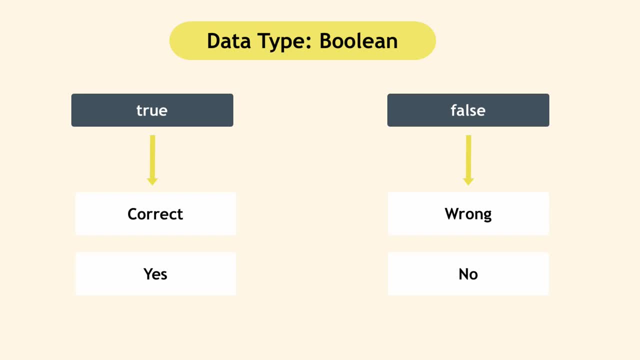 Is it a premium user? True, false. also Boolean expression, et cetera. Another data type is array that expresses lists. Think of applications that display List Lists of the same kind of data, like list of friends on Facebook or list of apartments on Airbnb or list of comments for your Instagram picture. lists have their own data types in all programming languages in JavaScript. 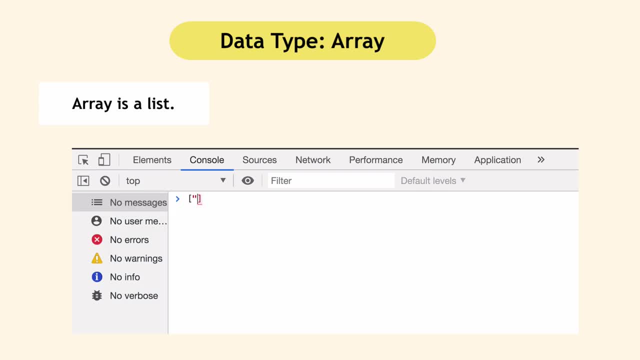 It's data type is an array. For example, list of friends names- will look like: this will be an array. that's an array that includes multiple names, And know the syntax of the array that encloses square brackets. So that's how JavaScript knows or can interpret that it's dealing with an array. 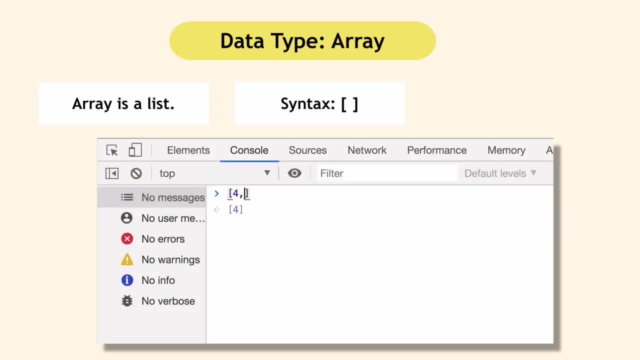 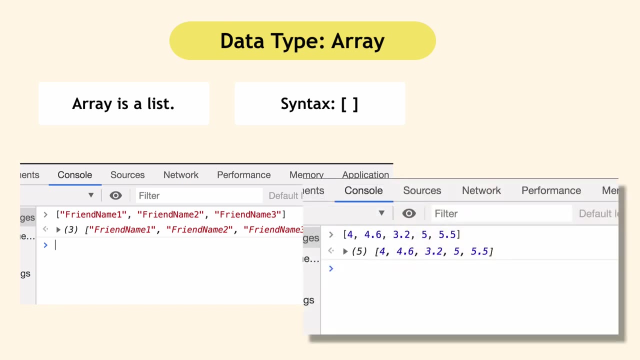 Or you could also have a list of ratings for Amazon products, for example. So this will be an array with numbers. as you see, array contains other data types. So here we have a list of strings and here we have numbers, And in JavaScript. 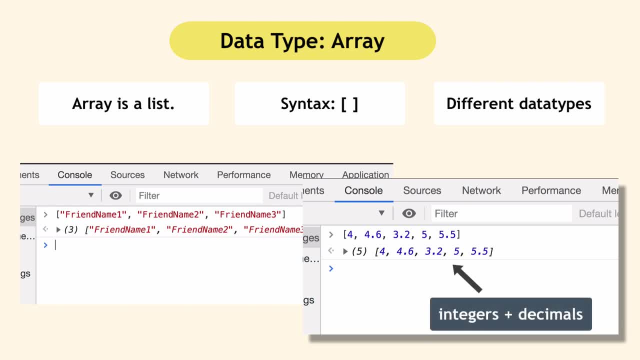 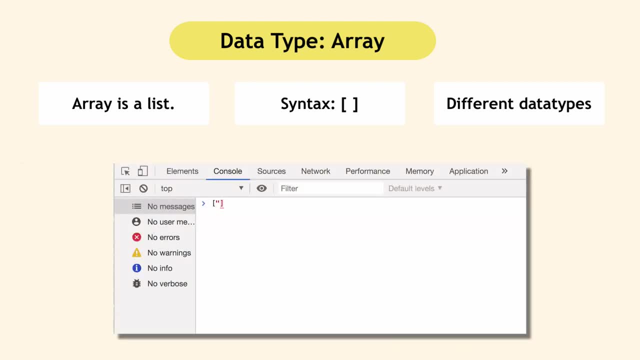 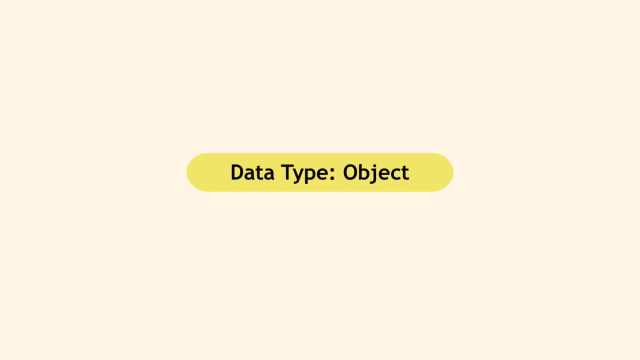 you can mix different data types inside an array. Here we have integers and decimals in one array. You can also write an array like this where you have string, integer and Boolean expression And the last data type in JavaScript is an object. Now in the Amazon review. 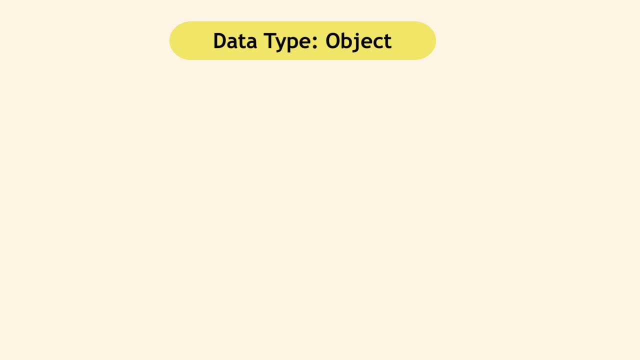 for example, you don't just see a list of ratings, You also see the author's name next to the rating and text they wrote in addition. So you need it. You need all this information grouped in one item in the array. You express that using object data type. 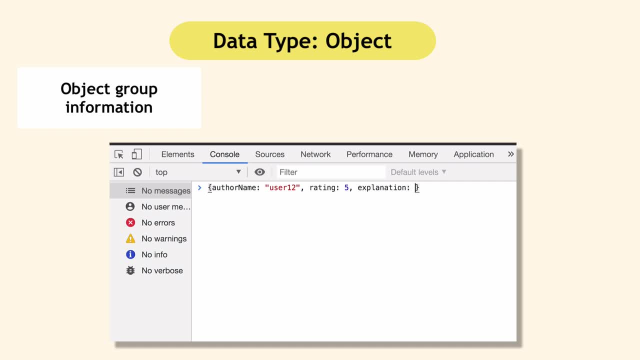 So a single rating object will look like this and note the syntax of curly braces. So, as we saw, array was expressed using square brackets and object is written using curly braces. So that syntax is important. So the JavaScript understands what data type you are writing. 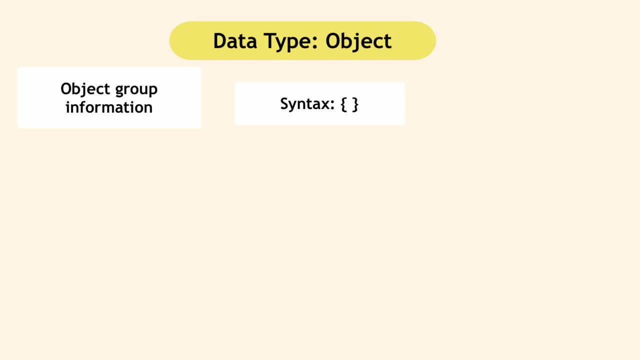 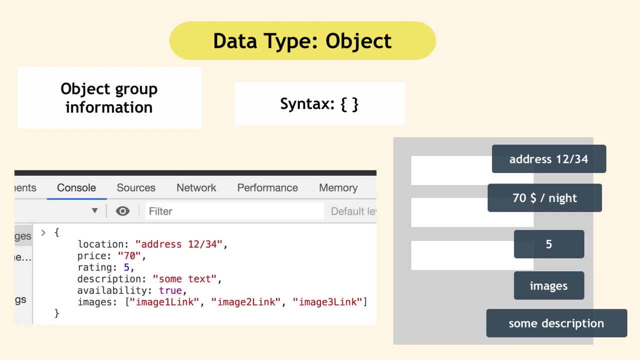 Another example is an apartment object on Airbnb which will include all the attributes it has, like location, price, ratings, description, availability, images, et cetera. So an object for that information will look something like this, just with more information inside. 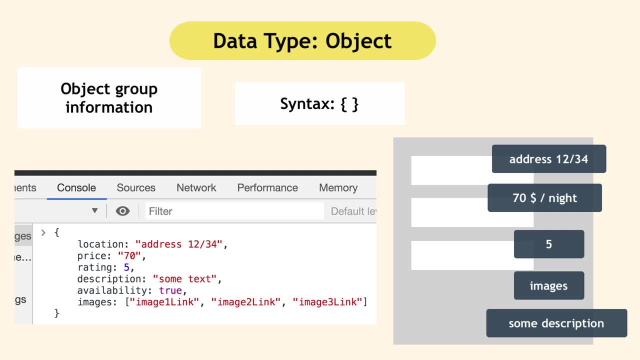 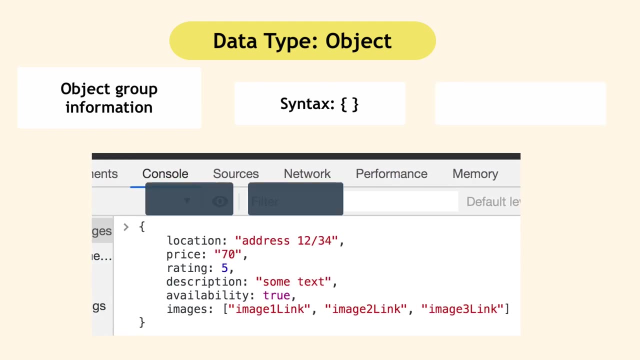 And here you see that the syntax highlighting of the browser is also helping to see that strings, Booleans and numbers are colored, Uh, in different way, meaning the JavaScript understands the difference between them. So, as you see, object has key value pairs, so that 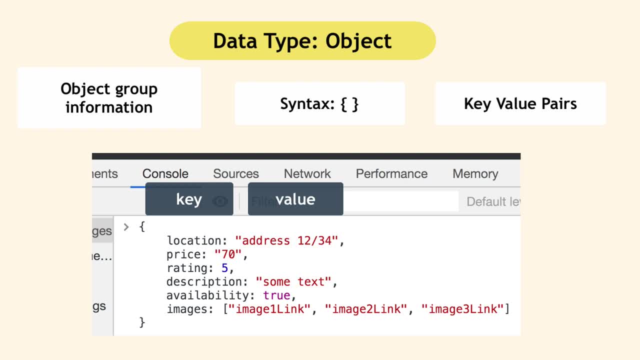 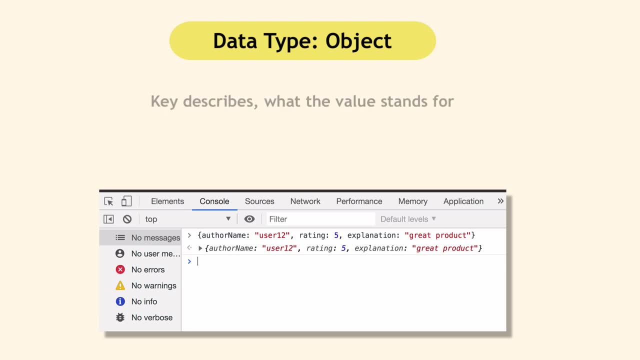 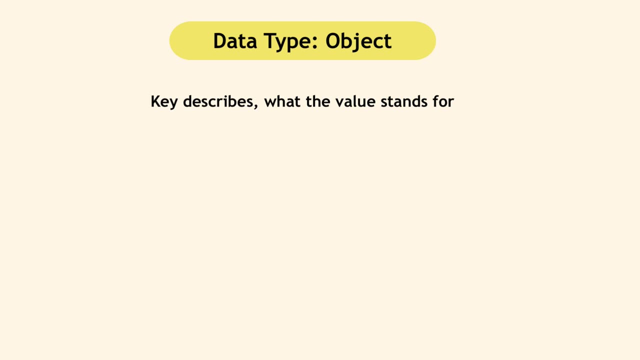 you know which value stands for what. So all these author name, user twelve, rating five- These are key value pairs where the key basically describes what the value stands for And the name of that key is totally up to you. You decide what that's going to be. 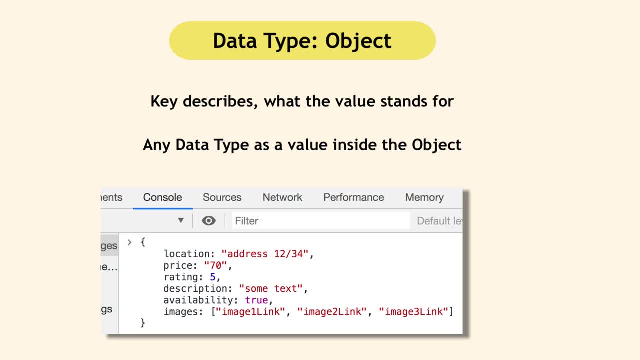 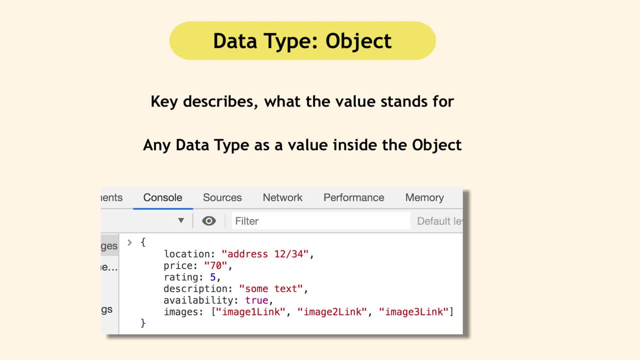 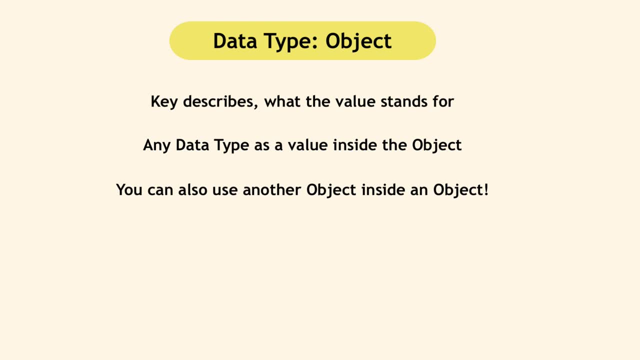 So here we have a string, integer, Boolean and array as a value, And you can also use another object as a value inside of an object. And finally we go back to the ratings. You will have multiple rating objects, so a list of rating objects. 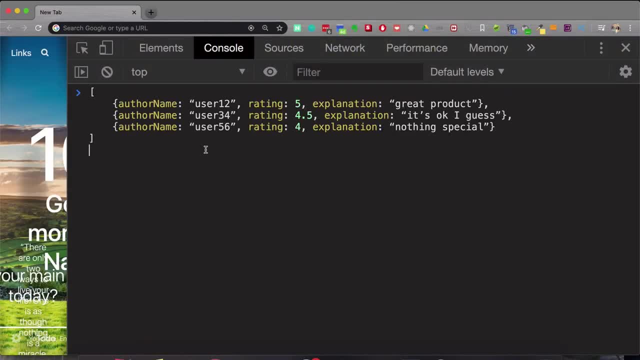 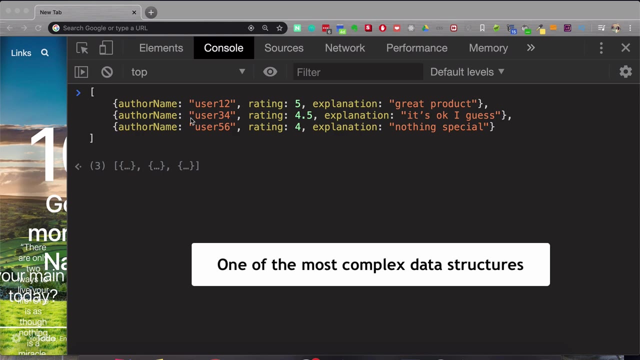 So the final list of these rating objects will look like this. So you will be an array with square brackets, and it will have a bunch of objects that are comma separated. Now, this is probably the most complex structure you will deal with most of the time. 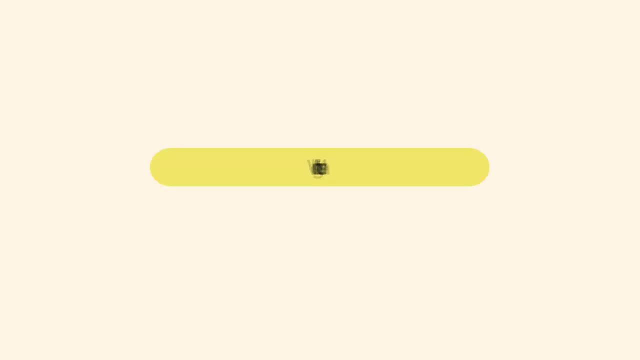 so it shouldn't get much more complex than this. Now we saw all this data type example values, but how do you use them to write a so-called logic? in JavaScript, The simplest use case is some basic addition, subtraction, et cetera. for numbers, 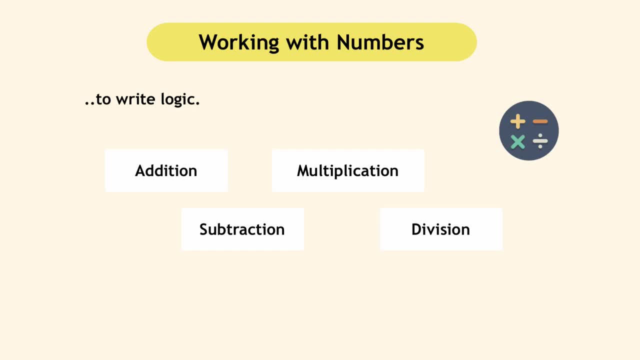 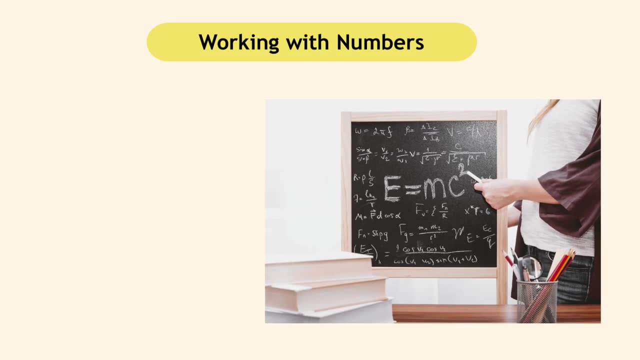 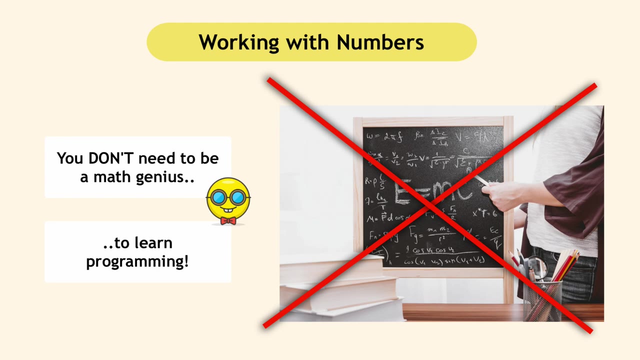 You can use simple arithmetic from element. It's cool to calculate basic things, And here I will use the chance to break this common misconception that you have to be super good at math to learn programming, which is completely, 100 percent wrong. I've been a software engineer for many years and I have worked in a lot of different projects and I have 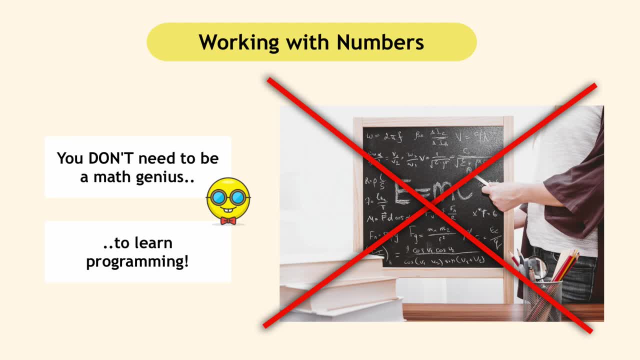 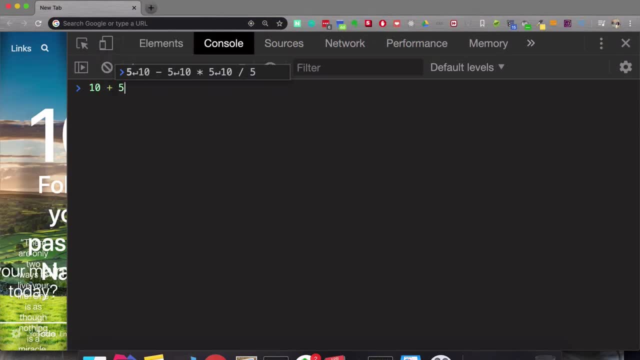 barely used anything more advanced than simple arithmetics like plus, minus, multiply and divide when writing web applications. So in JavaScript you can do all of this. You can do subtraction, multiply, divide, and you can also combine them just like you would with a calculator. 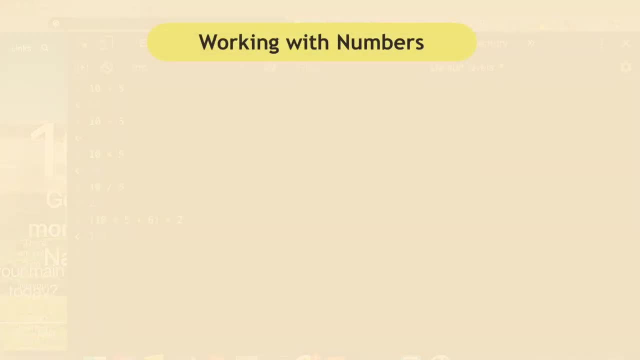 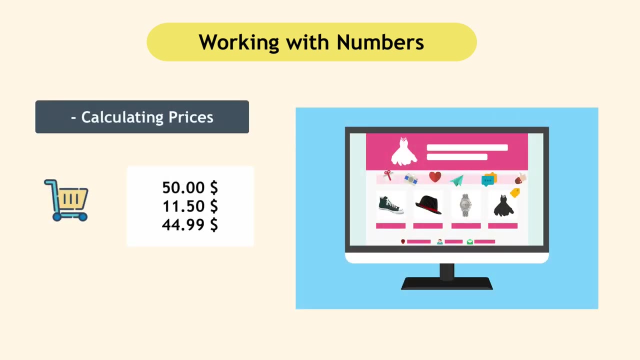 And, of course, you can do the same with decimals. Some real life use cases for these basic arithmetics are, for example, when you add multiple items to your shopping cart on Amazon, you see the sum and you also see the price breakdown, which is item prices plus shipment costs. 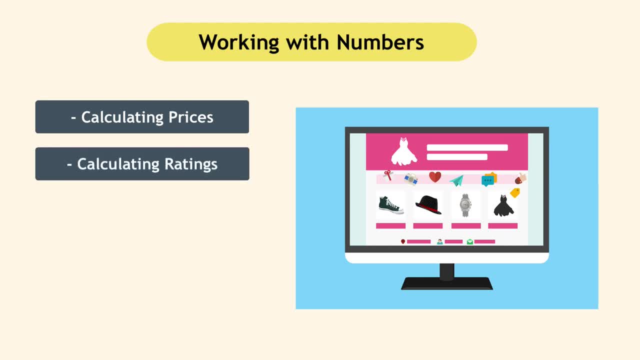 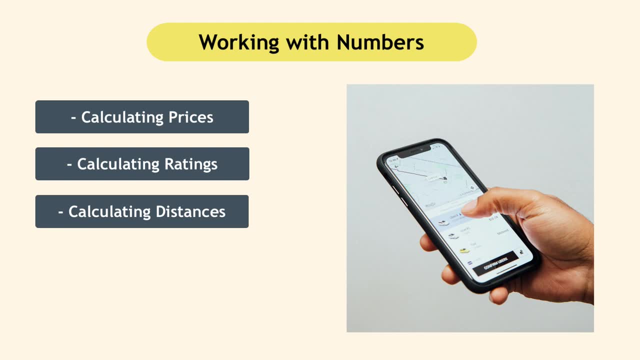 Or when you have product ratings, based on all the individual ratings, you display the average rating. or on Uber, For example, you see the distance from pick up locations to the destination in kilometers or miles and in minutes. All of these are simple calculations which are possible in JavaScript. 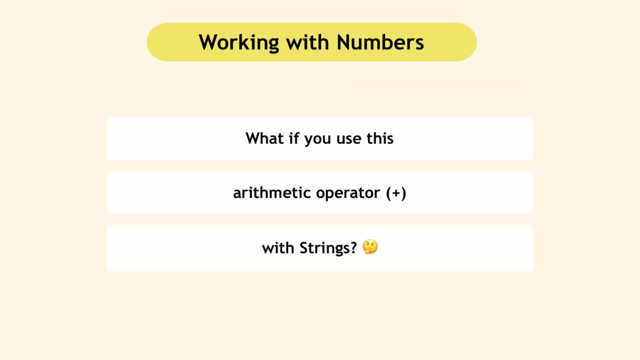 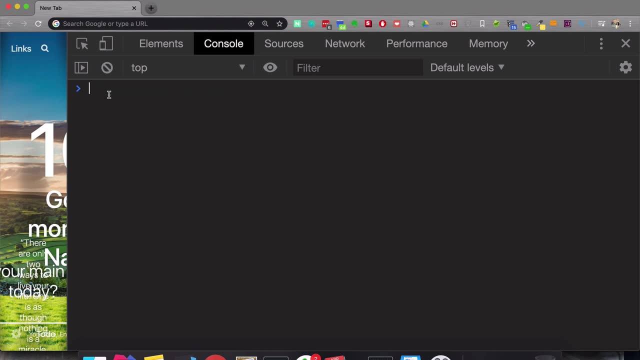 Now, obviously all these operators are meant for numbers, but there is a case where we can use the plus operator for string data types. So what will happen if I write string 12 plus string 12? So we get one thousand two hundred twelve. 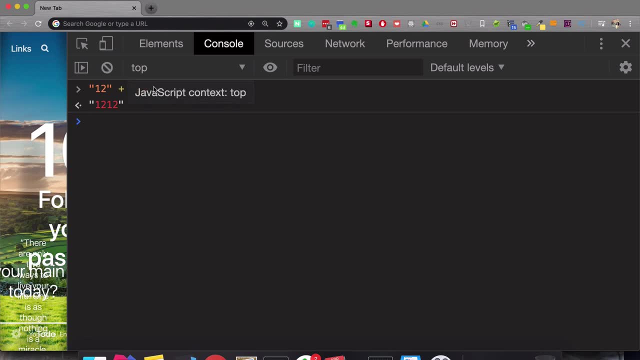 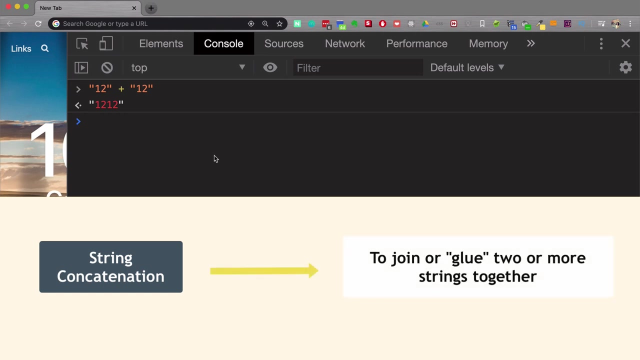 So what happened here is that JavaScript knows that these two are strings and not numbers, And instead of adding them, it handles them as strings by gluing them to each other, And in programing that's called string concatenation, And no, you don't have to remember that word. 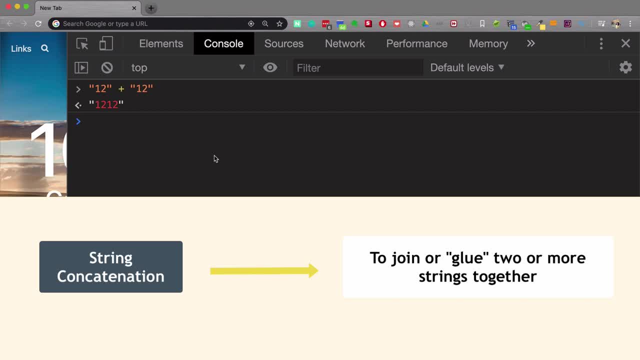 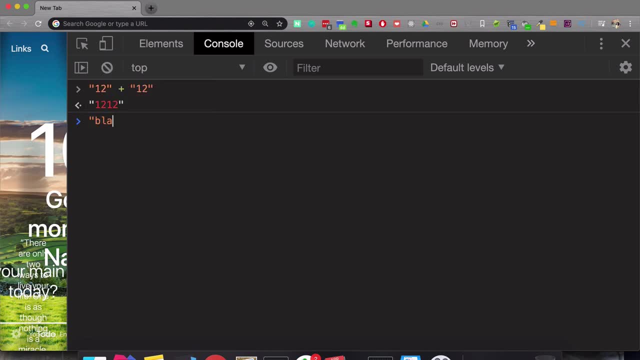 Just So you know that there are weird names for simple things in programing. the same way, you can glue a string to any other data type, So you can do blah to 12 and the number will also turn into a string, so to say. 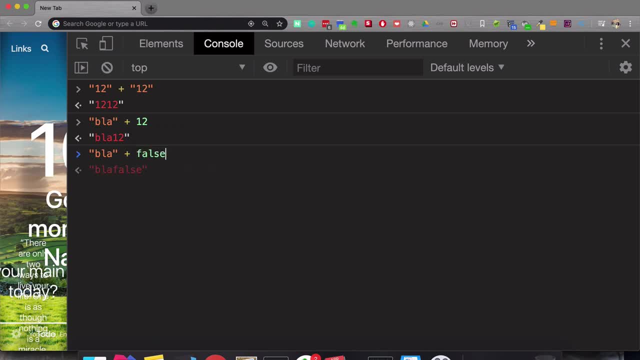 Or you can do the same with Boolean values, because JavaScript interprets that as you want to create another string out of these two values. And some examples probably don't make much sense, but in the next section of this video I will show you some more real life examples why this concept is actually very important. 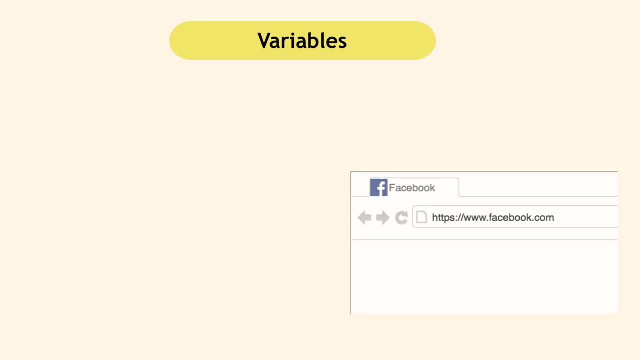 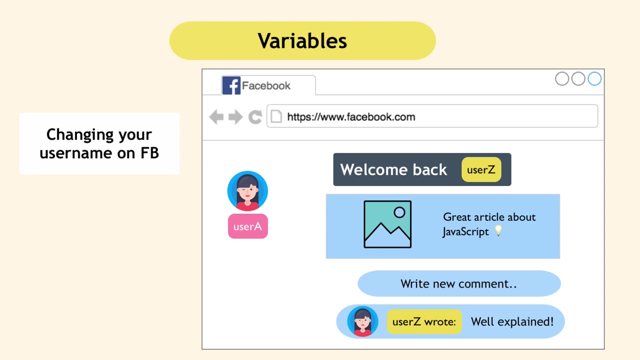 To understand the concept of variables, think about the following scenario: You change your username on Facebook, so obviously your changed username is displayed on your profile, but also all the comments that you wrote before the name change should now appear with your new username. 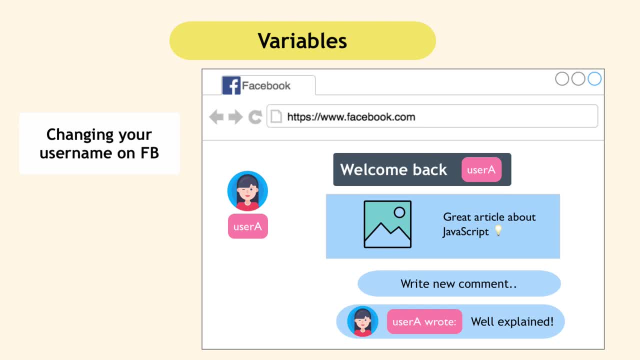 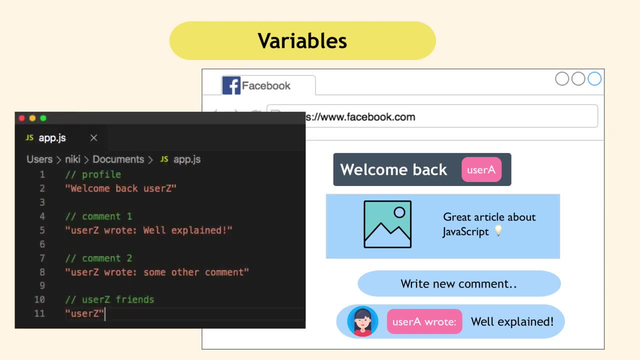 And also in all your friends lists your new username will appear Right. So this means if you had Facebook code where your username is written in all those different places, so you have your username in the profile section, you have your username in comment one, comment two, et cetera, and in all your friends lists. 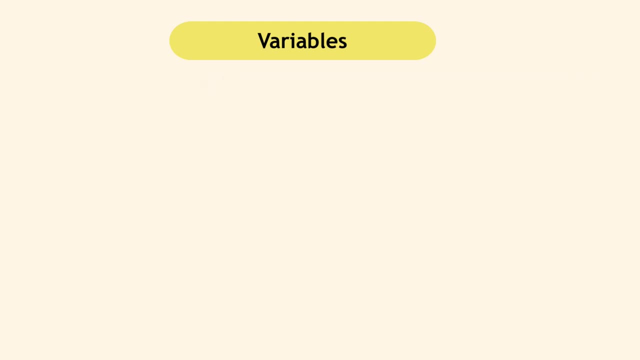 Right, Written directly, as is: Or. let's consider another example. Think about online shop. each product Has a price and it's displayed in a list in the product's own detail page and maybe also in combination to other products. So if the store now offers a discount and the price changes, obviously the price should be updated in each location where it's displayed. 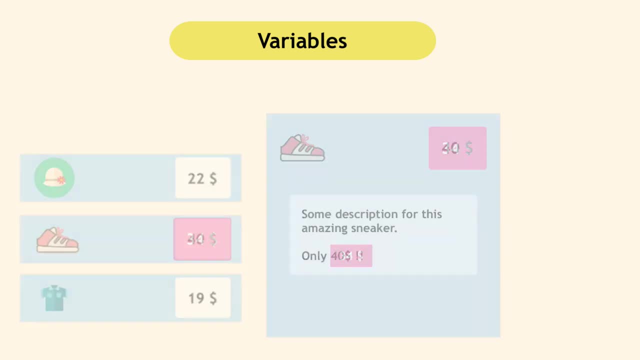 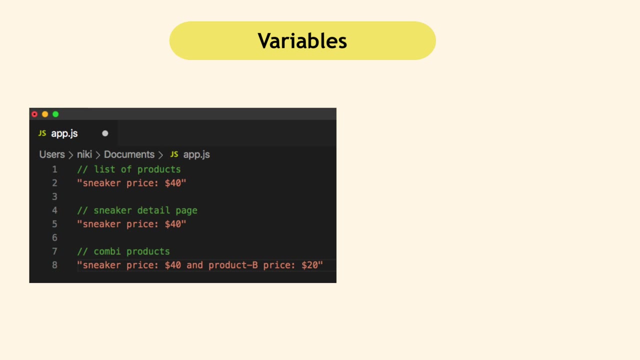 So again, in code it will look something like this. Obviously this is not a valid JavaScript code, but just to give you an idea. So somewhere in one JavaScript file you have the list of products where the product price is directly written, as is, and you'll have the same in detail page section of the product and combination. 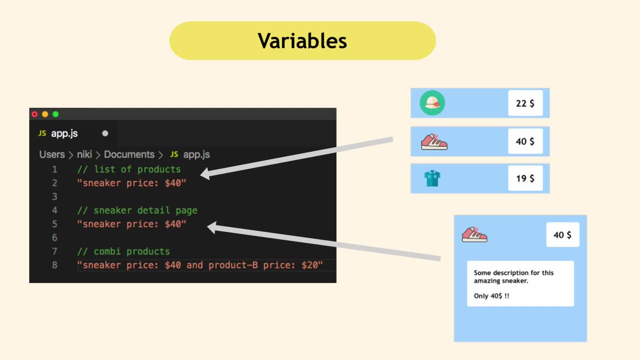 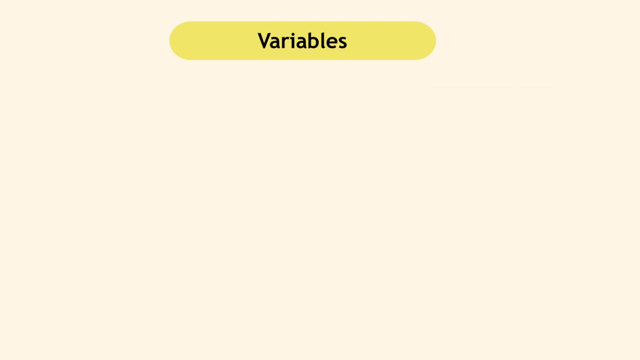 Now, when the username on product changes in those two scenarios, all these variables need to be overwritten, which means that you will have to go and change the price here and here and here and same with the username. Change it in all places where it's used now. 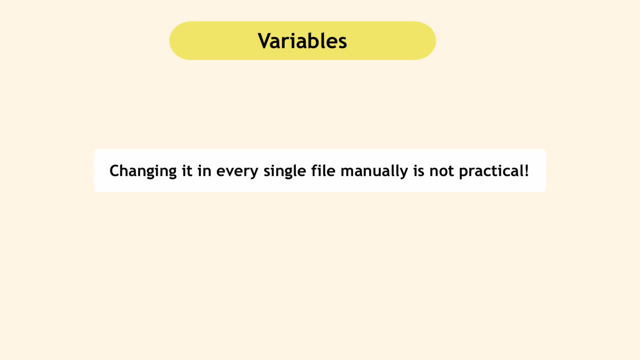 That would be absolutely inconvenient, considering applications are so dynamic and things change a lot, So that's where variables come in. So instead of writing the actual value in ten different places, you write the value once and then reference it ten times from ten different places. 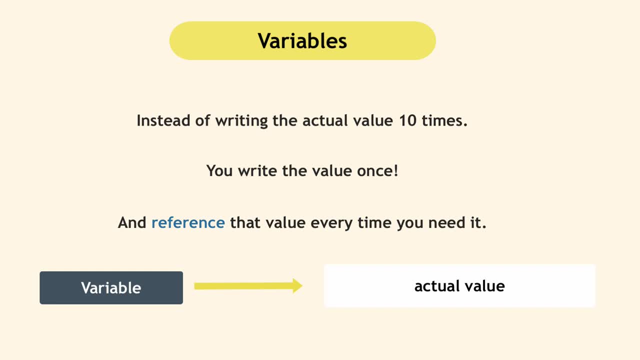 And that reference to the actual value is called a variable. and you give variables a name That makes sense For that value. So, for example, product a price equals fifty. So now you create a reference for the value 50, which is called product a price or username equals abuser eight. 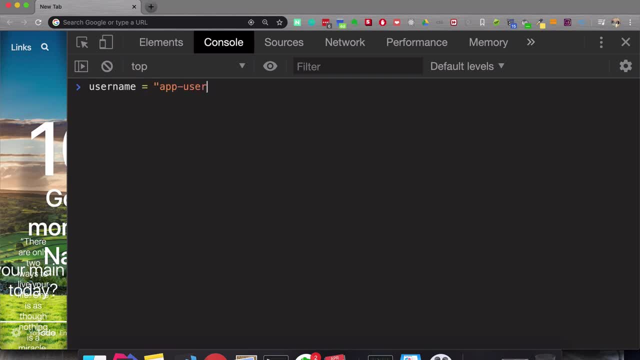 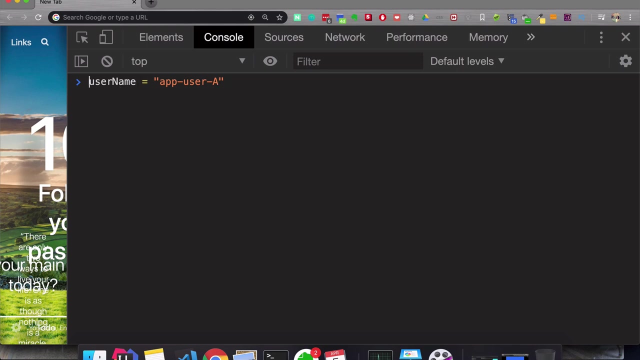 So you take the actual value, which is string, and create a reference to it, But in addition to that, you should also let JavaScript know explicitly that this random name that you just came up with is a, a variable, and you do that using a VAR keyword. this and remember, keywords are words that. 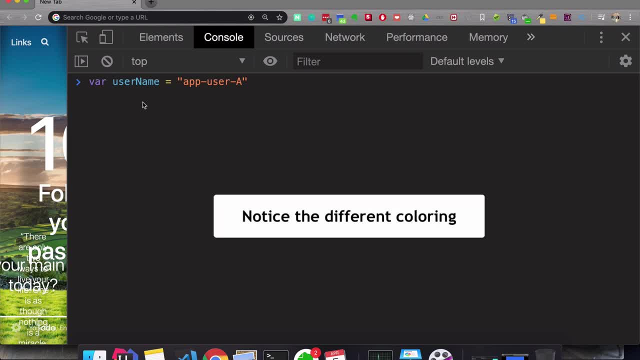 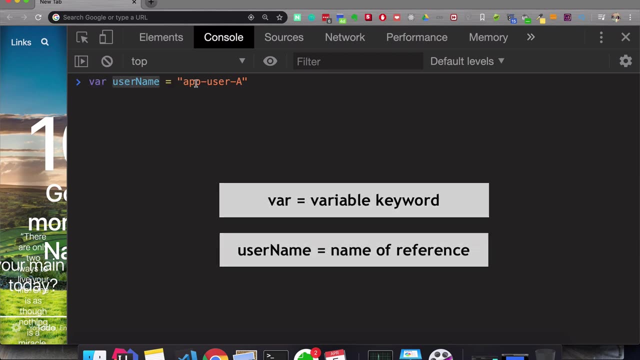 have special meaning to JavaScript And because of that, if you noticed, the coloring or the highlighting of the word changed once I added VAR in front of it. So now JavaScript knows that this is a variable keyword and this is the name of that reference or variable, or. 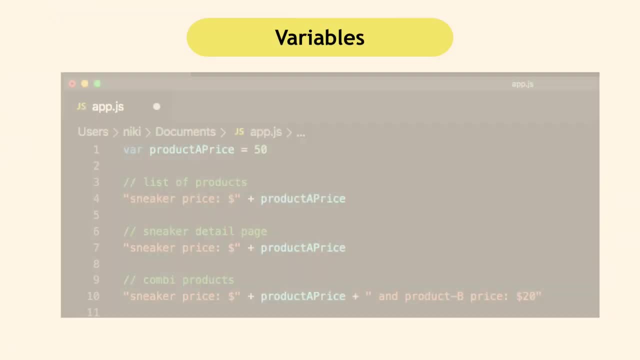 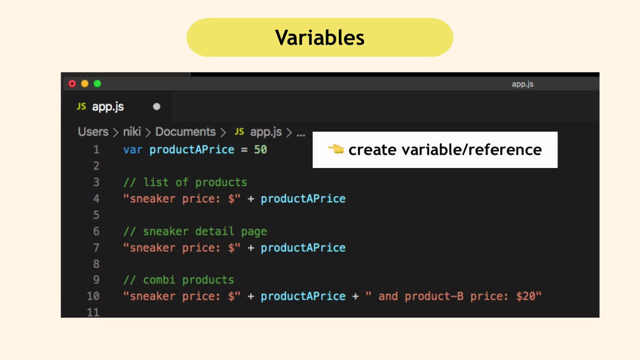 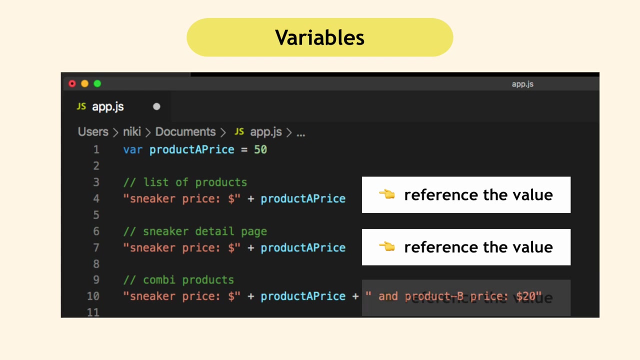 the same with product, a price variable, and in cold it will now look like this. So first you'll create that reference somewhere like this, and then in all the locations or all the places in JavaScript code where you need that value, that actual number value you. 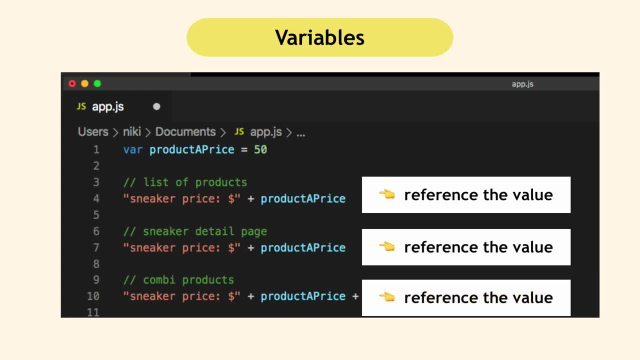 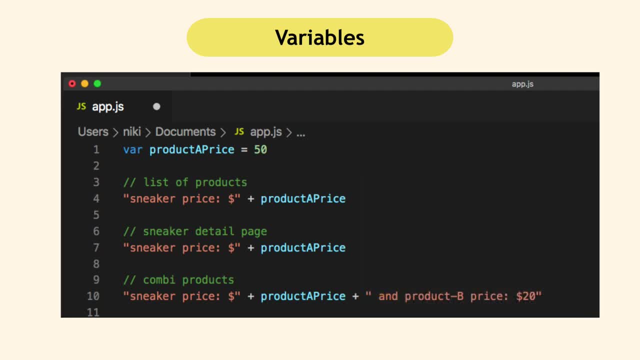 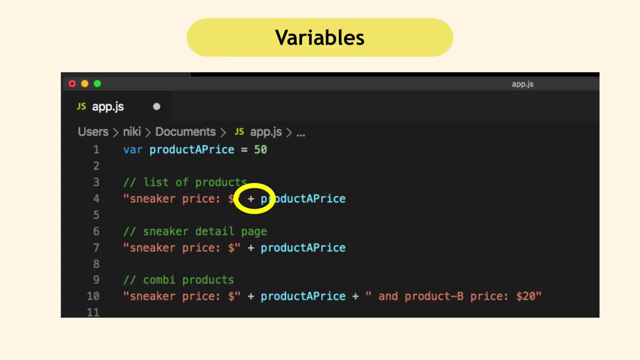 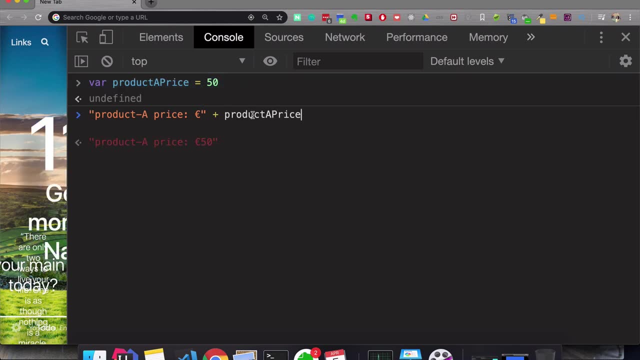 that I showed you earlier. this is an example of string concatenation, meaning string is glued to another value, And this is where this concept is very useful. So when you run or execute this line, what happens is that JavaScript in the background replaces this. 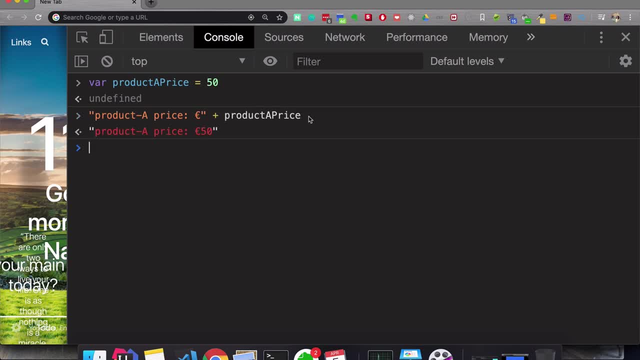 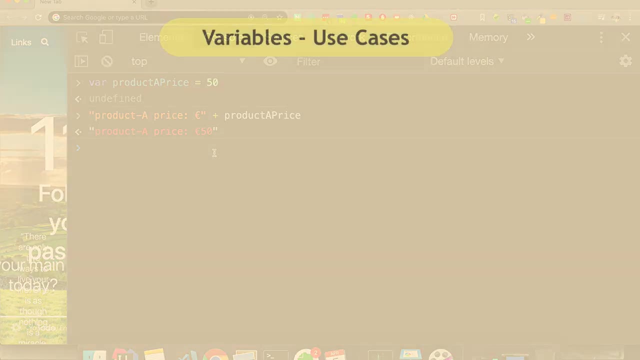 reference with the actual value. So when I execute this, I see product a price 50. And this is a real example where plus operator with strings is actually very important And you will use this a lot because you will use variables a lot in order to make this variable. 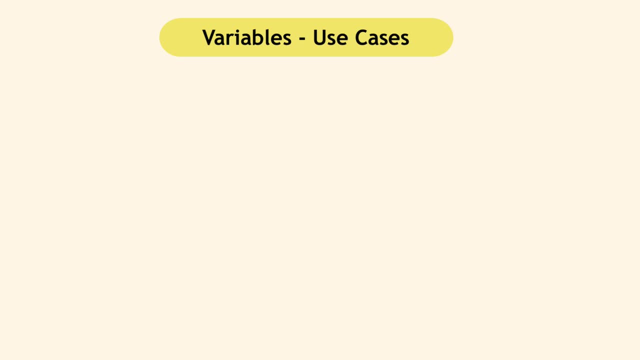 concept stick more. Let's consider two additional use cases. First, consider multi language applications. on most applications, You can select a preferred language and see all your navigation buttons, et cetera, in your language. Now, if the application supports ten, 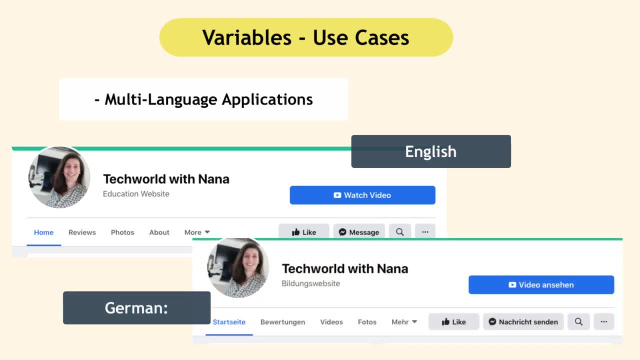 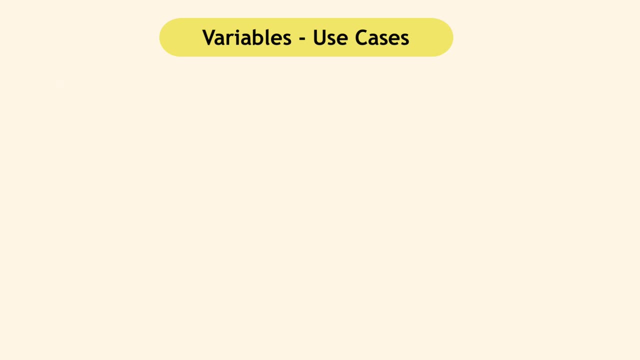 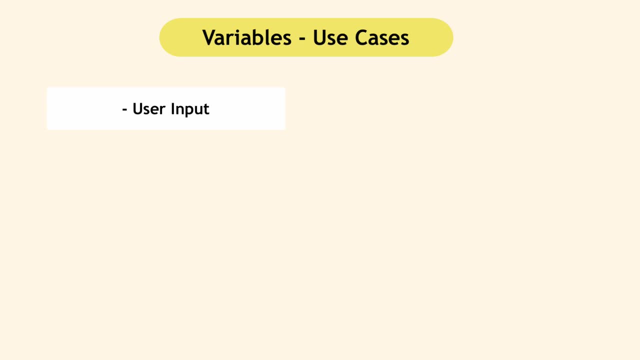 use case, which is very important, is user input. So when you sign up for a web application, you need to enter your name, last name, email password. These are all user inputs. So what you input in the application as a developer when you, when you prepare that. 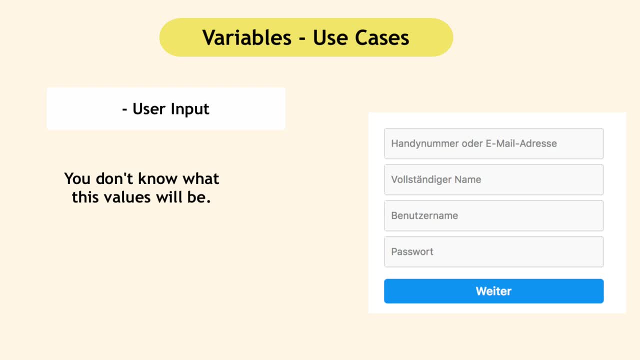 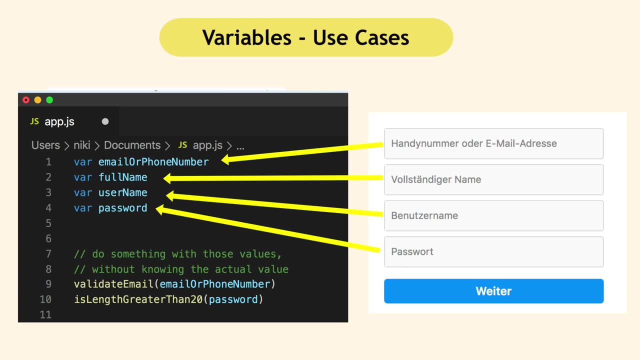 code for future usage. you don't know what these values are going to be, because users can enter anything, But what you know is the name of the variables that will reference these values, And this way you can use the actual values without even knowing what they. 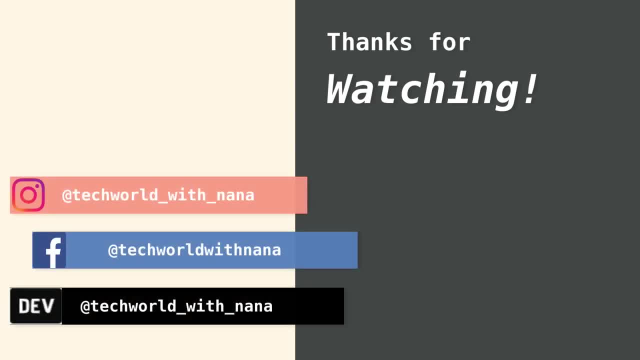 are Now. if you want to practice these concepts so that you can remember them better, in the description of this video I will link some websites where you can do Practical exercises on the JavaScript concepts that I explain in my videos.